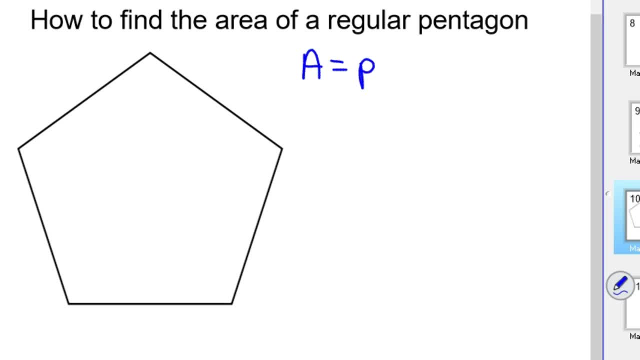 Area of a regular pentagon is the perimeter, and this is any regular polygon- is the perimeter times apothem, and I'll explain what an apothem is here in just a second, All divided by 2.. So in our case, so let's say this thing is 12 meters, This is a pretty good sized pentagon. 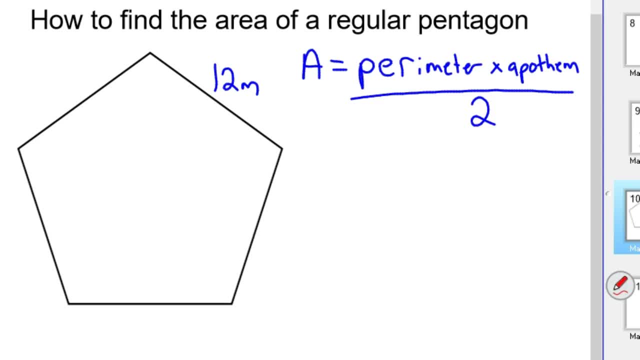 And we've got this 12 meter pentagon. All the sides are 12 meters. then What I like to do, and what many do, is you split this up into regular triangles Where you connect the center to the radii or to the vertices. 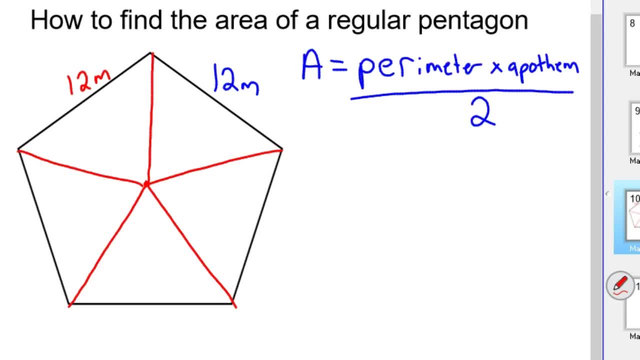 To create radii. So those red lines are the radii. The apothem I'm talking about is the height of each of those triangles. They're all the same triangle and they're all congruent, but this blue line is the apothem. 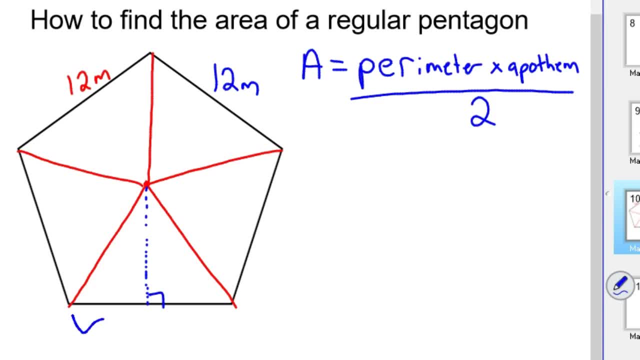 And so once you have that apothem- because we've already got the base and I'll go ahead and use the formula, since I've spewed it out there- So it's 12 centimeters. well, 12 times 5 is 60.. 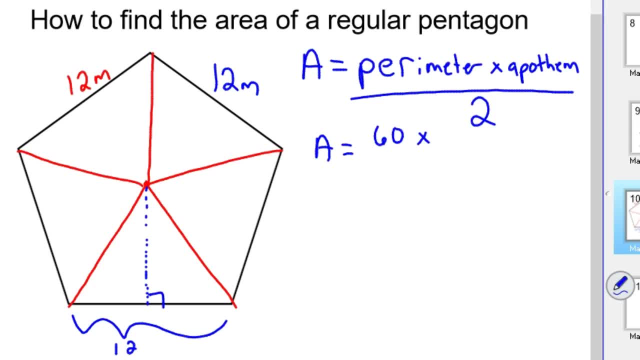 So we've got most of this formula created here 60 times. I'll call that apothem. A divided by 2 is all we have left to find. is that apothem. So let's go ahead and find this thing. 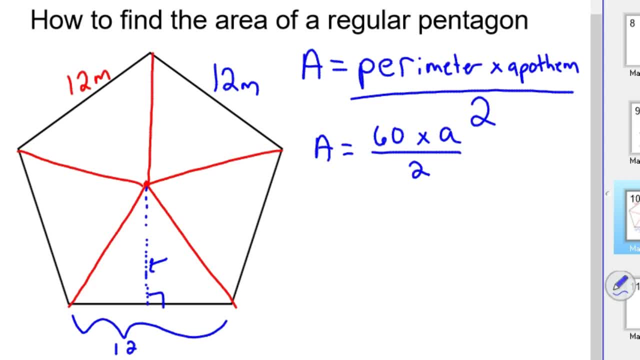 Well, we're going to need a little more information. Well, first off, we divided the pentagon into triangles, And so each of these angles all the way around makes a circle. If you add them all up, you'd get 360.. 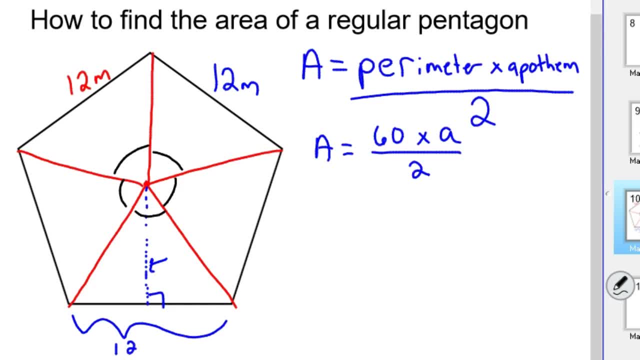 Well, there's 5 of them, So 360.. So 360 divided by 5 is 72.. So that's 72 degrees And we're going to split that in half with the apothem here, So this angle is just 36 degrees. 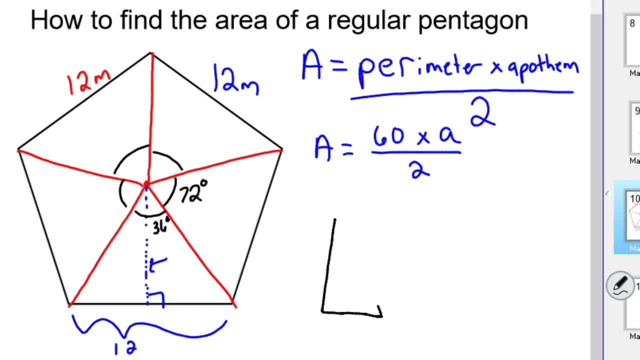 So we could pull that triangle apart. You know this length. here is half of the 12, which is 6, which would go here. Here's my 90 degree angle. Here's my apothem. Here's my 36 degree angle. 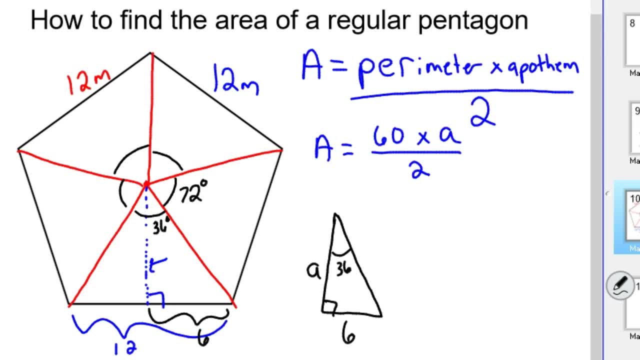 And so we're really ready to solve this And we're going to have to use trig in this case. So 6 is opposite, A is adjacent, The radius is hypotenuse. We don't really need it for the area, but I'll put it in there anyway. 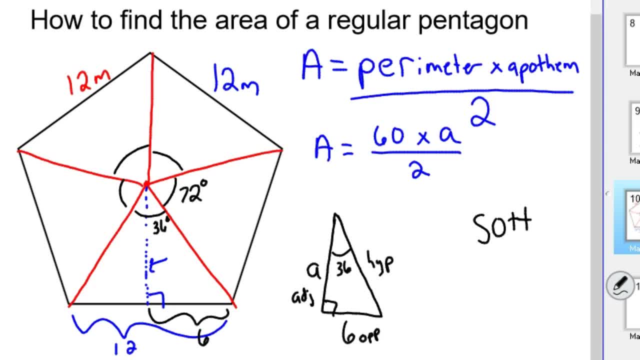 And if you remember SOHCAHTOA S-O-H-C-A-H-T-O-A, You know we've got the opposite. We're looking for the adjacent. Well, the only one dealing with opposite and adjacent is tangent. So we're going to use tangent in this case. 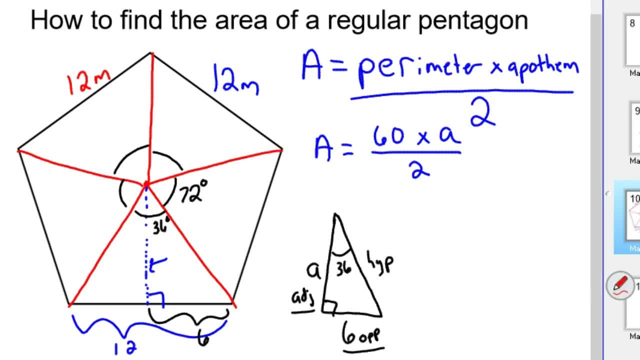 So tangent 36 degrees is equal to opposite over adjacent, which is 6 over A. So I always like to use the Google calculator. I have my kids use that as well. So we're going to go tangent 36 degrees. 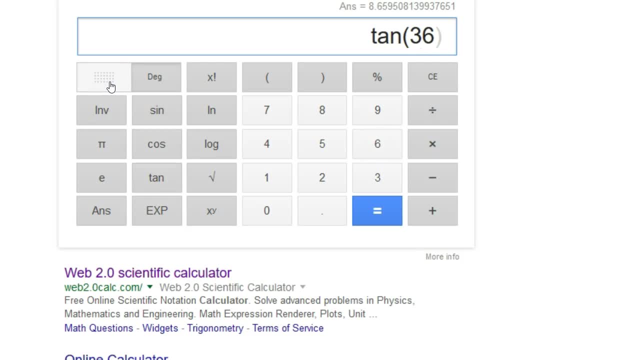 Make sure you know that's radians, that's degrees. Make sure you convert that to degrees first. In this particular case, we're not messing with radians yet, So tangent 36 is .7265.. And we'll just round that. 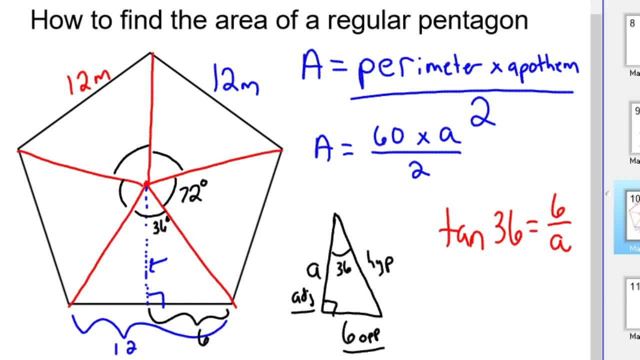 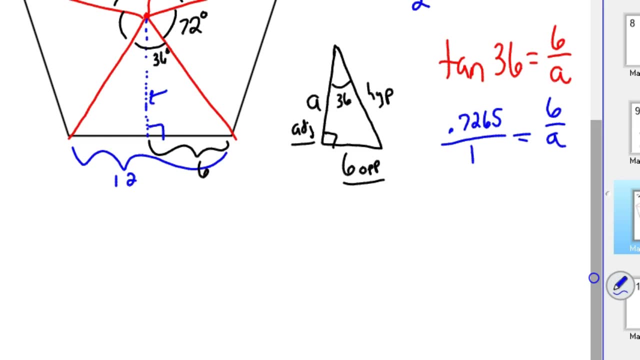 Keep that .7265.. And we'll put that over 1.. That's in place of the tangent 36.. Equals 6 over A, And then we'll cross multiply. And so if you cross multiply that would be .7265 times A. 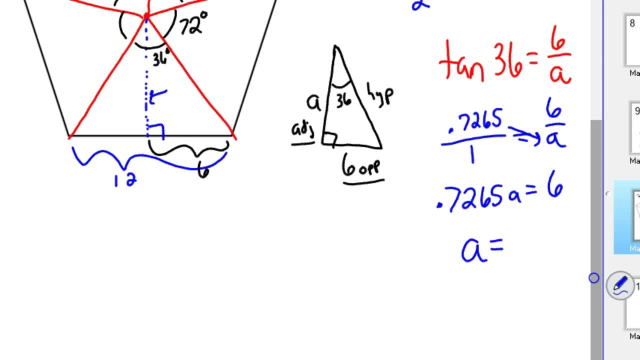 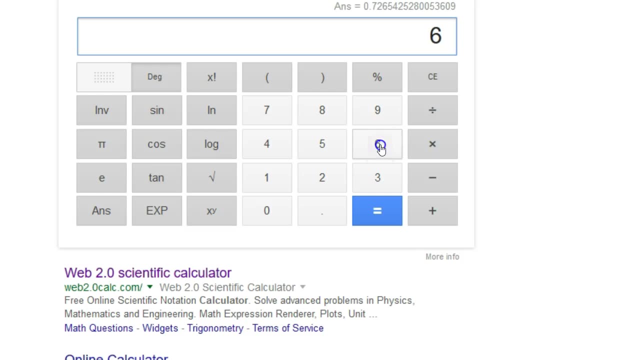 Equals 6 times 1.. So we know A or the apothem- or apothem, I think, is how they say. that is 6 divided by .7265.. So back to our calculator. So 6 divided by your previous answer is 8.26..